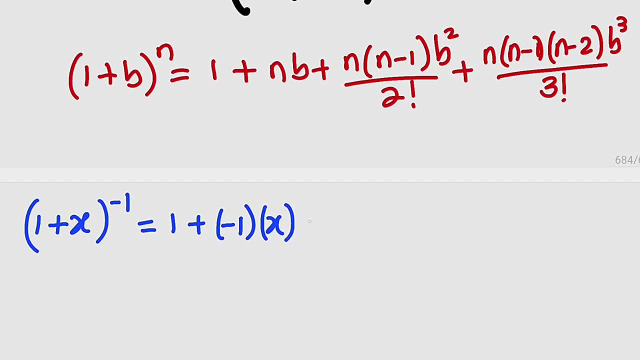 multiplied by b, which is x. We move to the third term: plus n, which is negative, 1, multiplied by n, which is negative 1.. Minus 1 again, then b squared, that is x squared divided by 2 factorial. then the last term, that 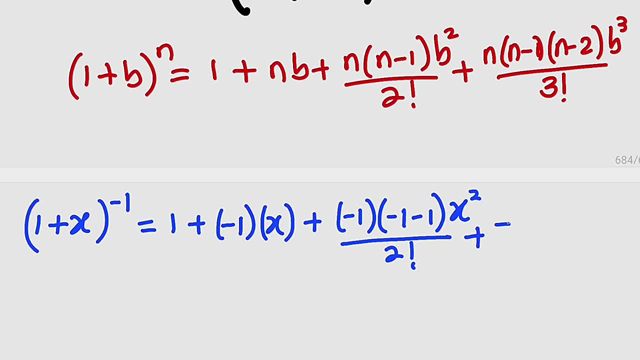 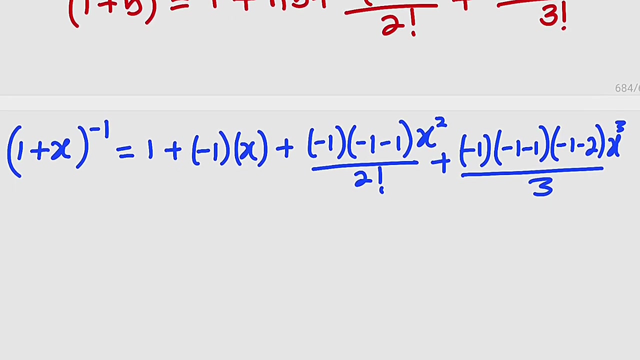 we are looking for will be plus n, which is negative, 1, multiplied by negative 1 minus 1. multiplied by negative 1 minus 2, then x. to the power of what? 3, then divided by 3, factorial. Alright. so now let us simplify and get our final answer: This is equal to 1.. If you multiply these, 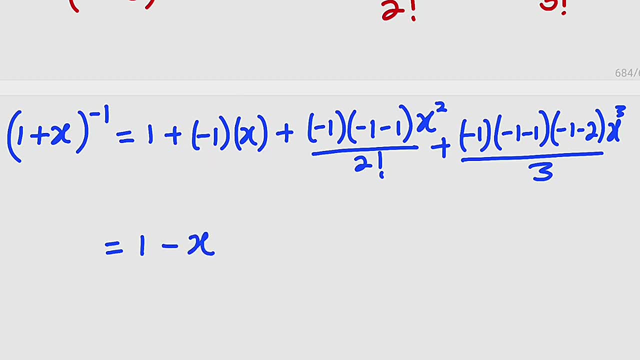 two together, you have negative x. Then we move to the other terms. We have negative 1. negative 1 is negative 2.. That negative 2 multiplied by negative 1 will give us positive 2 multiplied by x squared. So we have positive 2 multiplied by x squared, divided by 2 factorial, which is 2.. 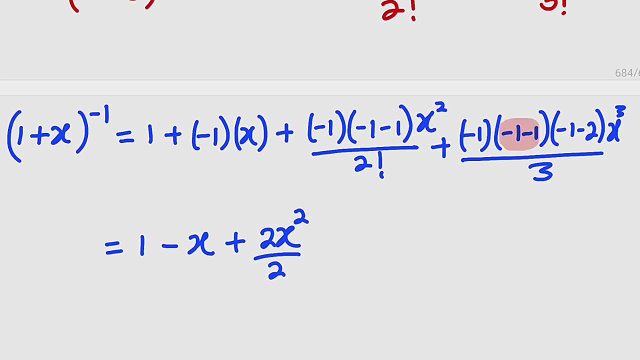 Then the last one: Negative 1. negative 1 is negative 2.. So we have negative 2.. Let me write it here. Then we have negative 1, negative 2, which is negative 3. If you multiply this by negative 3, you have: 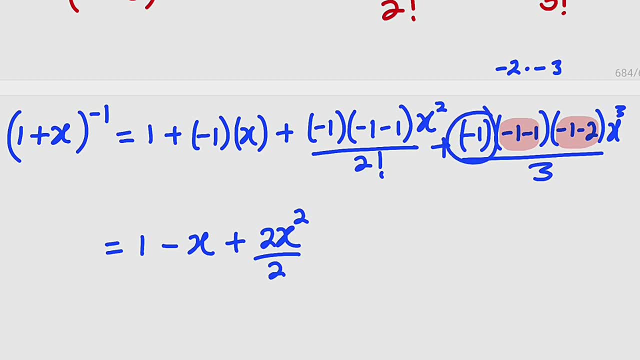 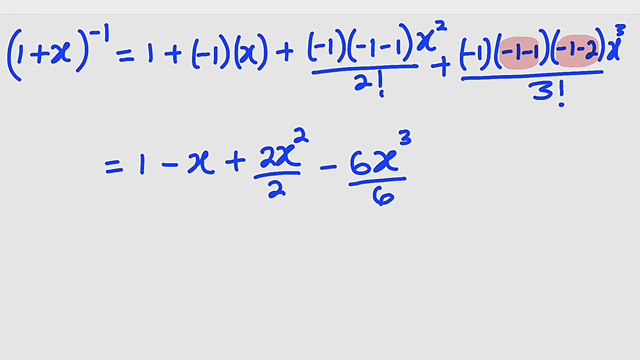 positive 6, and that positive 6 multiplied by negative 1 will give us negative 6.. So we have negative 6. x to the third power divided by 3 factorial. Sorry, this is 3 factorial and 3 factorial is 6, right? So we can simplify this as 1 minus x plus this 2 will cancel this 2, right? So we have 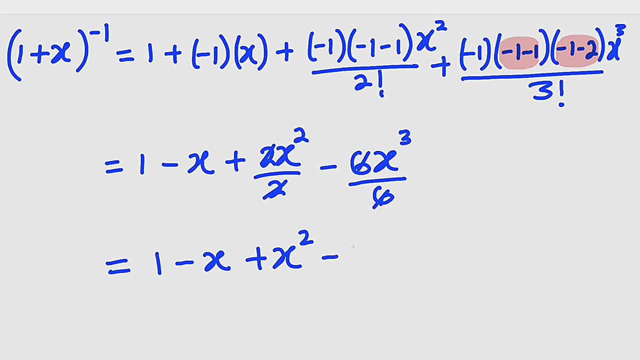 x squared, This 6 will cancel this 1.. So we have minus x to the third power. Remember that this is what 1 plus x raised to the power of negative 1.. This is just the first four terms We have.